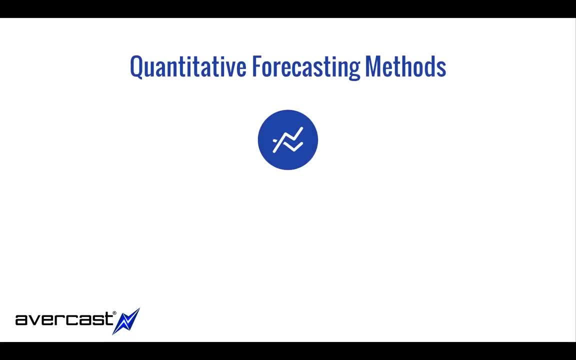 different approaches And so as we look at quantitative forecasting methods, we can really break that out into these four approaches, Or these four approaches are what we commonly see. There are groups that use the naive approach, which is really just looking at what happened in the previous period and saying that's going to happen again. right, I sold 100. 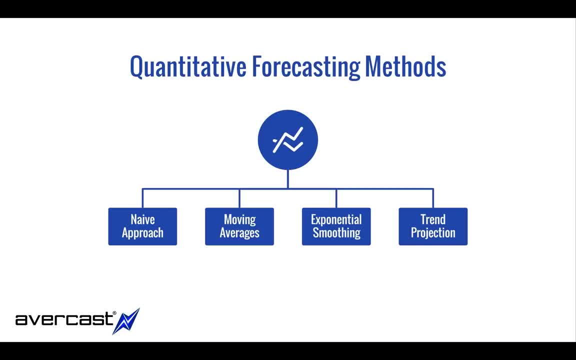 widgets last period, this period I'm going to sell 100 widgets again. Moving averages might say, okay, the last three periods. if I take the average of what happened in the last three periods, the next period will probably be the same as those, And then we kind of move that average along. 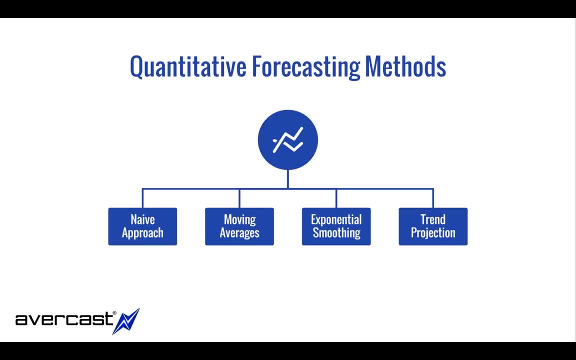 whether it's three periods, six periods, 12 periods. Exponential smoothing basically goes, And it's really a matter of taking a weighted average approach when we're looking at these moving averages. So we're going to weight different periods differently because maybe they're more relevant to the forecast, And so it's a little bit. 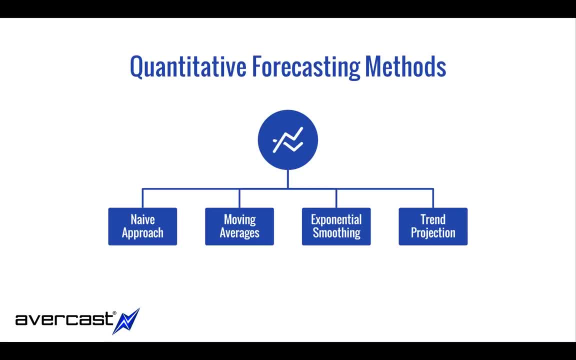 more robust and a little more sophisticated when we're talking about forecasting methods. And then, of course, there's trend projection, where we look at what is the trajectory of what's happening. Maybe we're increasing every single day, and sometimes every 10 days. maybe it's not happening. 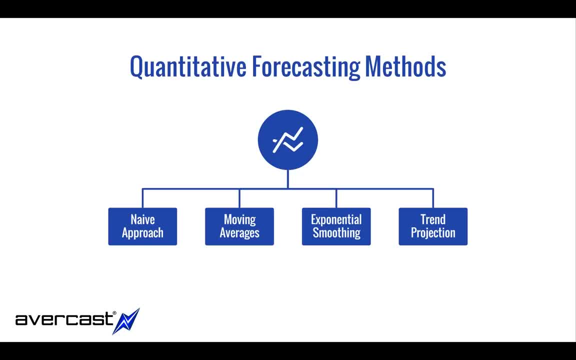 every single period, or we've had like two increases, a small decrease and then another increase, and so we see, you know, we're starting to see this rise or this increasing trend, and so we need to take a look at that, And so we'll look at. 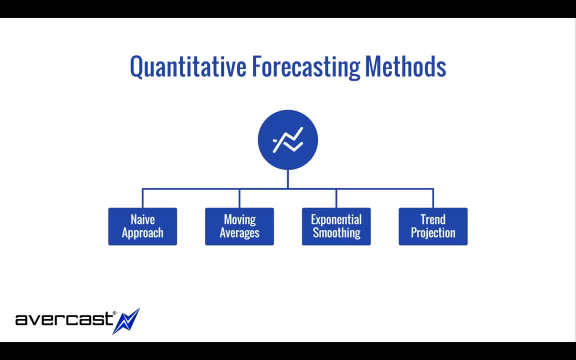 those, and then we'll also throw in a bonus, a bonus video where we'll talk a little bit about linear regression and then how to think about that and perhaps even dive in deep a little bit on some of those things. The qualitative forecasting methods. there are four of those that we'll cover as 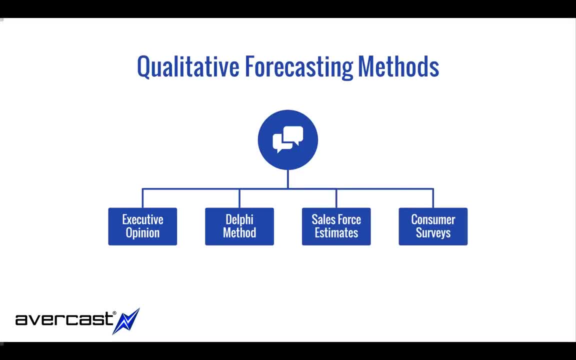 well, There's executive opinion, which is typically, when we're looking at a group of executives, that they're going to make a decision or an opinion about what's going to happen in the next period. You've got the Delphi model method, which 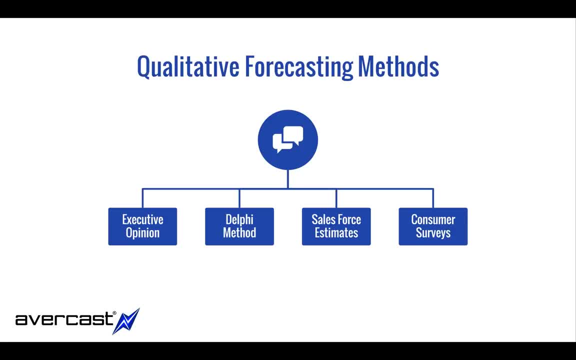 is where you've got consumers that- or maybe they're just trusted advisors or something like that- but they give their opinion about what they think is going to happen, how many widgets they'd buy, or how many widgets they think would be sold in different markets or wherever else, And then you've got.